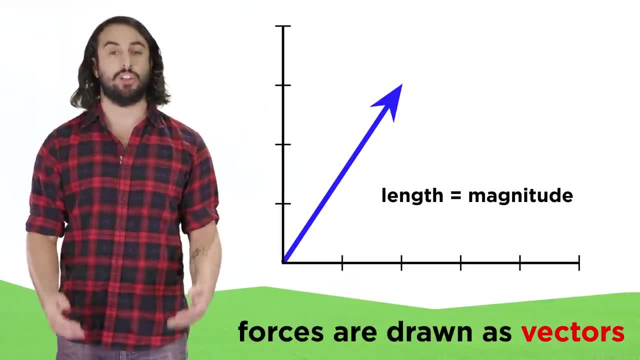 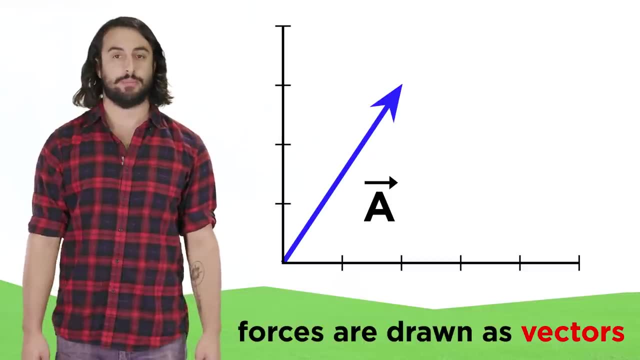 They will not be represented by the length of the arrow, which will indicate the magnitude of the vector. To denote vectors, we usually use letters in bold font with an arrow on top. As we learn more about physics, we will use vectors to predict the motion of objects. 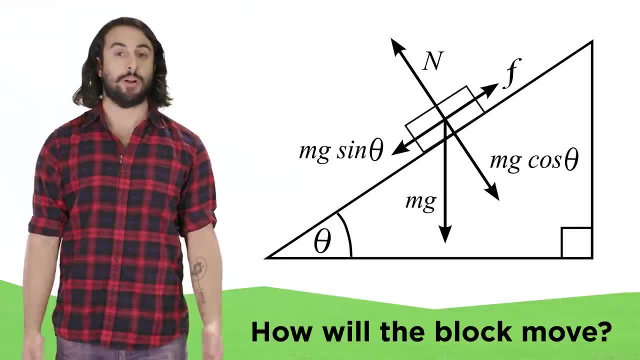 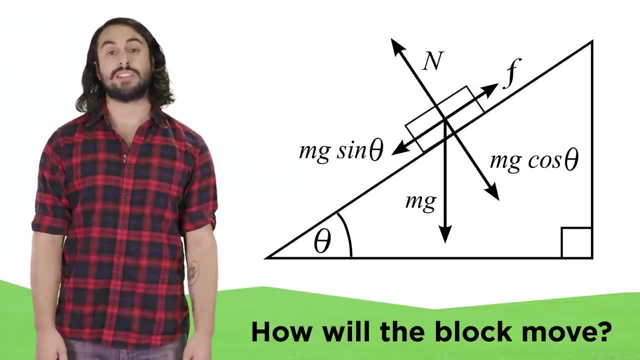 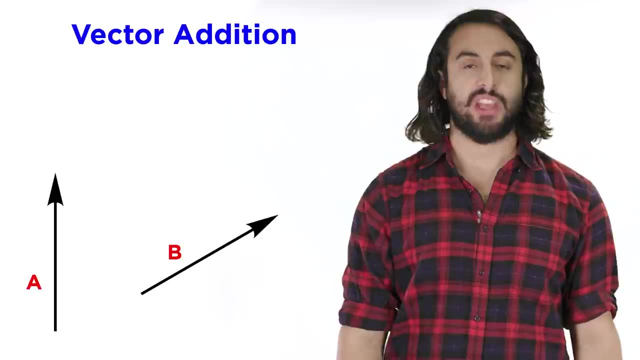 and if there are several forces acting on an object, as there often are, we will need to be able to do certain operations with vectors in order to perform our calculations. so let's learn how to do simple vector operations. If we want to add two vectors together, it's pretty simple. 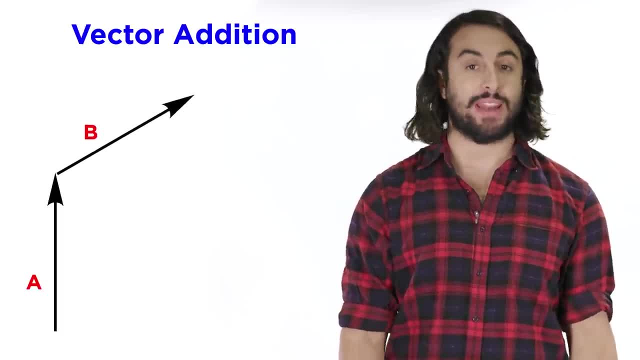 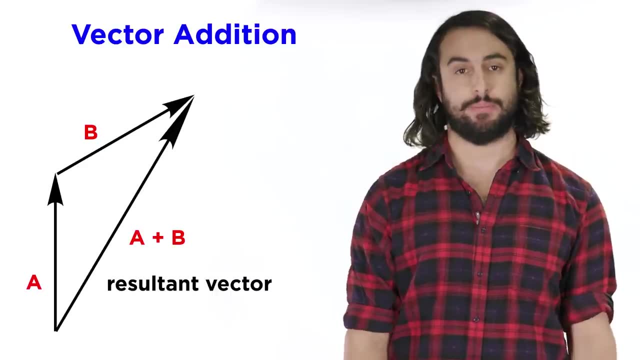 We just make the second vector start where the first vector ends and then create a new resultant vector that goes from the start of the first to the end of the second. In lining up two vectors, we have to make sure they retain their direction as that. 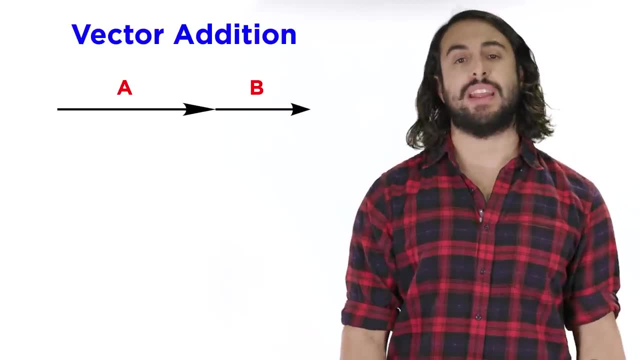 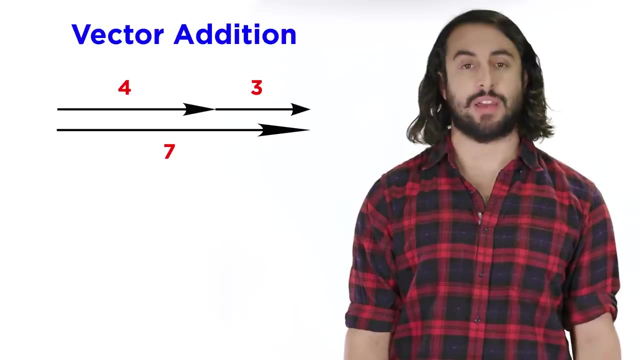 is important information. If the vectors point in the same direction, their sum will just be a longer vector and the magnitude of this resultant vector will simply be the sum of the magnitudes of the original vectors. so in this case, four plus three equals seven. 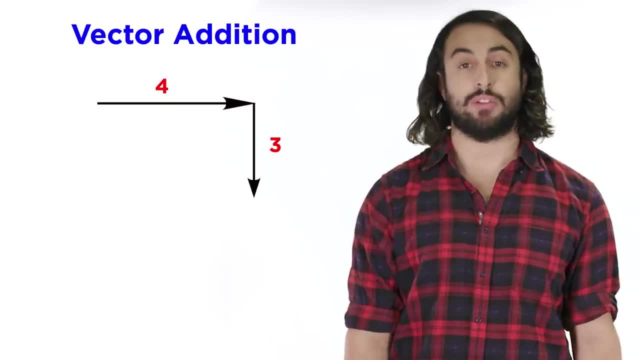 Sometimes there is an angle between the two vectors, like these perpendicular vectors. In this case, when we draw the resultant vector, it will be the hypotenuse of a right triangle. The magnitude of this resultant vector will be functions of the same type. 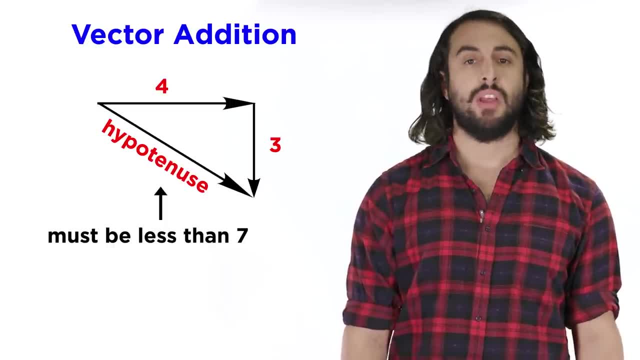 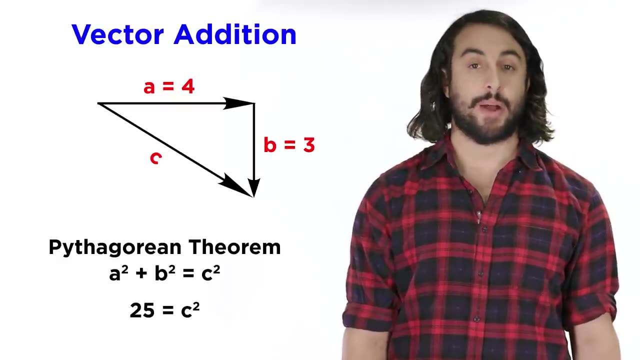 we are missing Meaning vector is not the sum of the other two magnitudes. This one can be found by using the Pythagorean theorem which we may remember from algebra: class A squared plus B squared equals C squared. Plug in A and B, square them and find the sum, and then we take the square root to get. 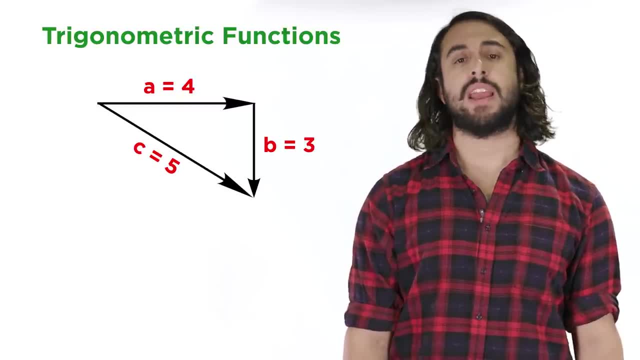 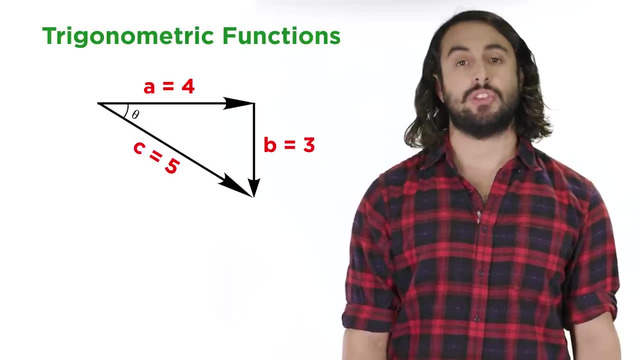 C, which in this case will be five. When we are looking at right triangles, we can also use trigonometric functions to find the unknown angles. All we need to do is choose an angle which we represent with the Greek letter theta. 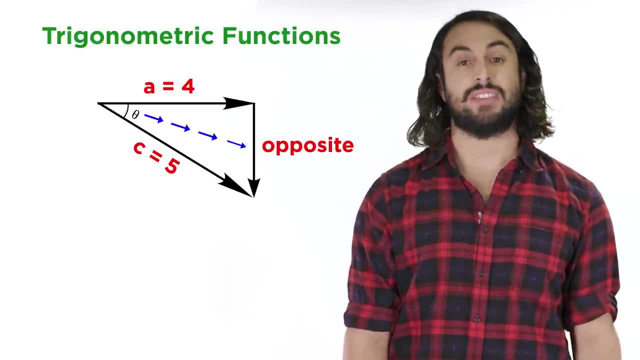 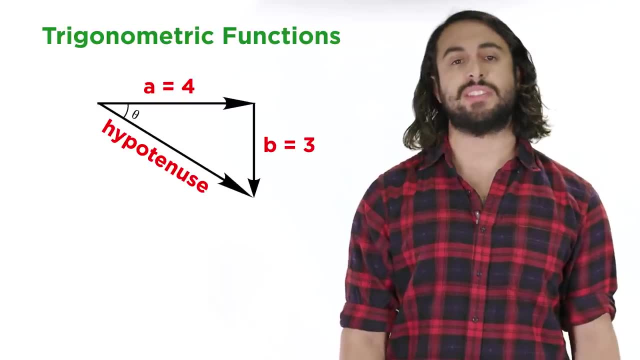 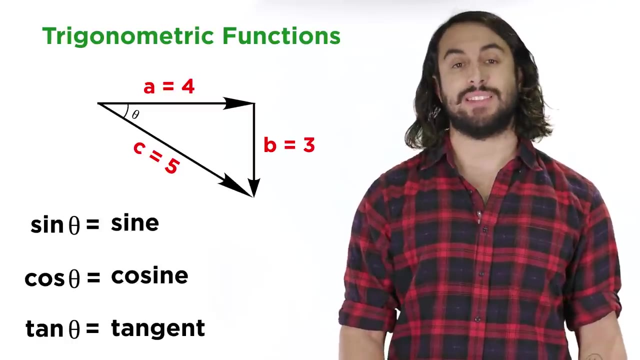 and label the sides of the triangle as opposite: the leg directly opposite the angle adjacent the leg right next to the angle and the hypotenuse, which is always the longest side. We can use the lengths of these sides to find the sine cosine and tangent of this angle. 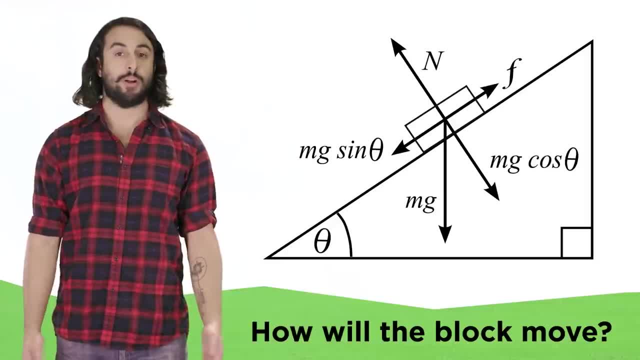 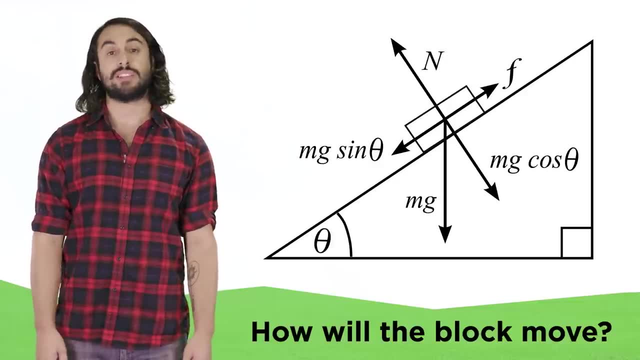 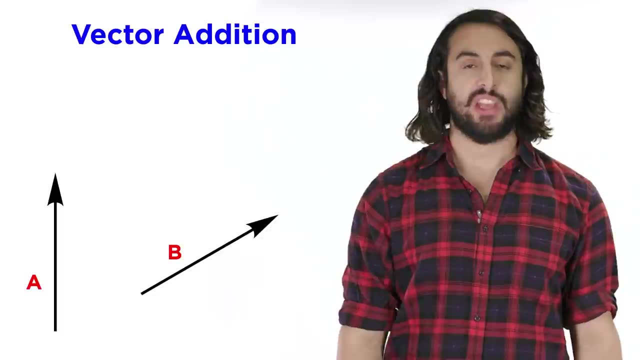 and if there are several forces acting on an object, as there often are, we will need to be able to do certain operations with vectors in order to perform our calculations. So let's learn how to do simple vector operations. If we want to add two vectors together, it's pretty simple. 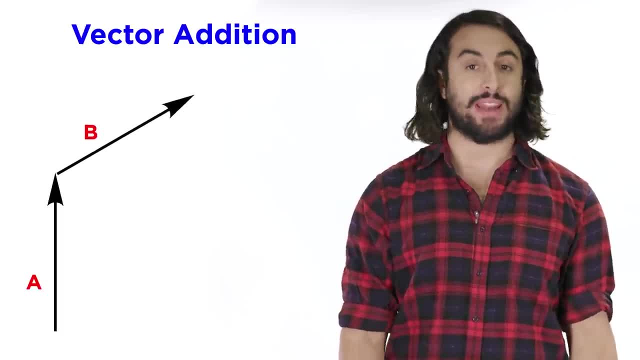 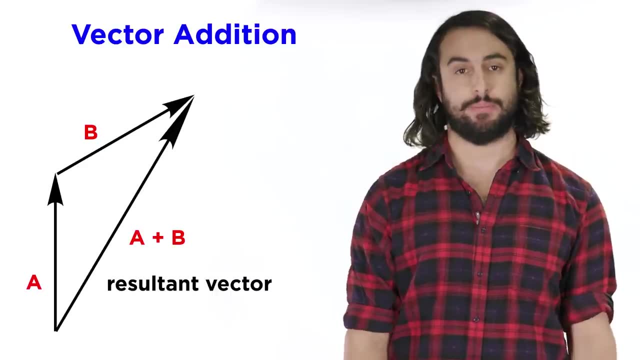 We just make the second vector start where the first vector ends and then create a new resultant vector that goes from the start of the first to the end of the second. In lining up two vectors, we have to make sure they retain their direction as that. 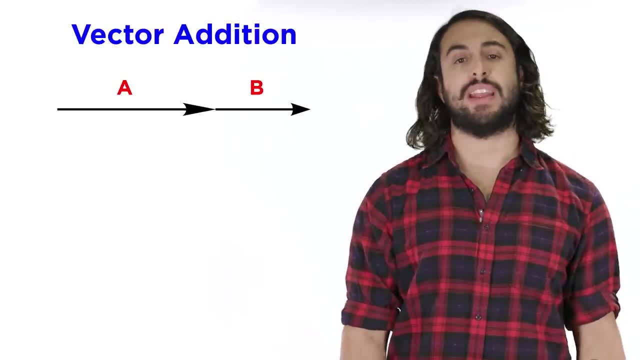 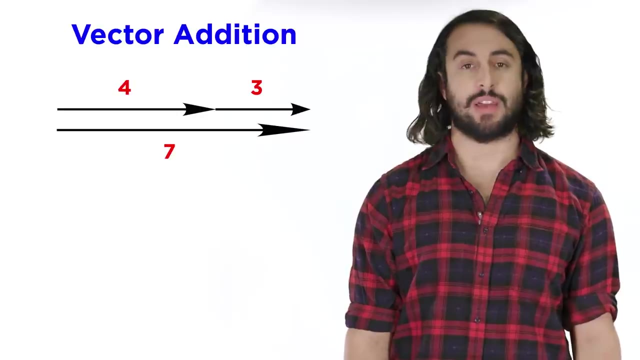 is important information. If the vectors point in the same direction, their sum will just be a longer vector and the magnitude of this resultant vector will simply be the sum of the magnitudes of the original vectors. So in this case, four plus three equals seven. 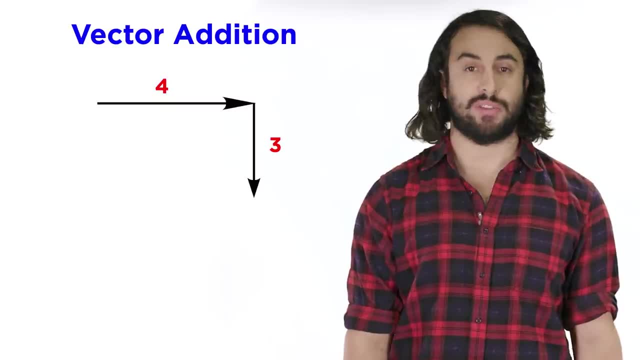 Sometimes there is an angle between the two vectors, like these perpendicular vectors. In this case, when we draw the resultant vector, it will be the hypotenuse of a right triangle. The magnitude of this resultant vector will be equal to the magnitude of the resultant. 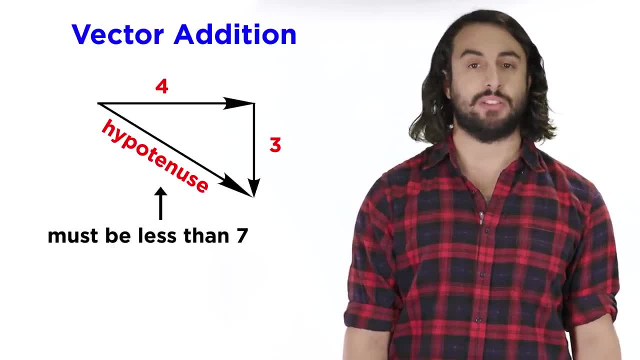 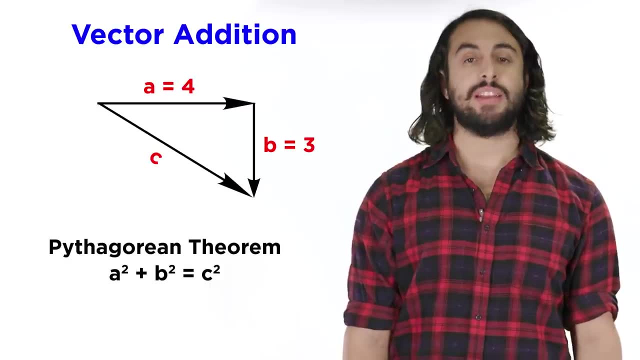 vector. vector is not the sum of the other two magnitudes. This one can be found by using the Pythagorean theorem which we may remember from algebra: class A squared plus B squared equals C squared. Plug in A and B, square them and find the sum, and then we take the square root to get. 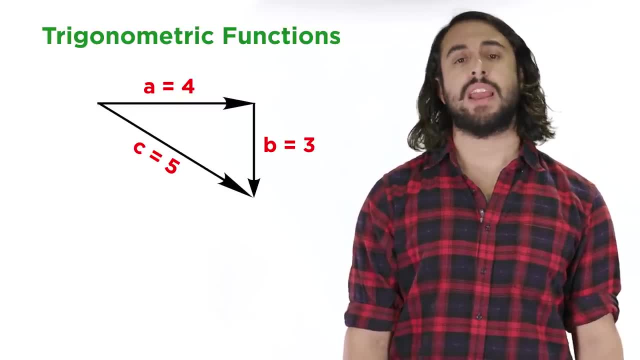 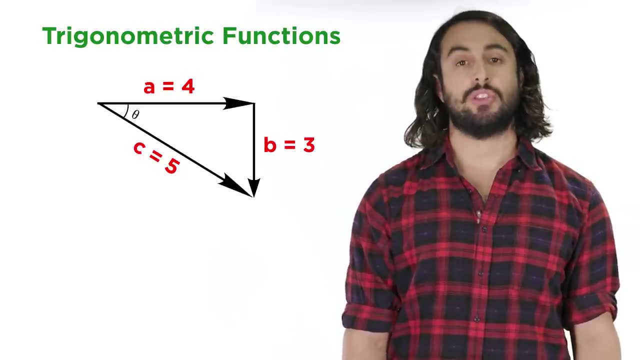 C, which in this case will be five. When we are looking at right triangles, we can also use trigonometric functions to find the unknown angles. All we need to do is choose an angle which we represent with the Greek letter theta. 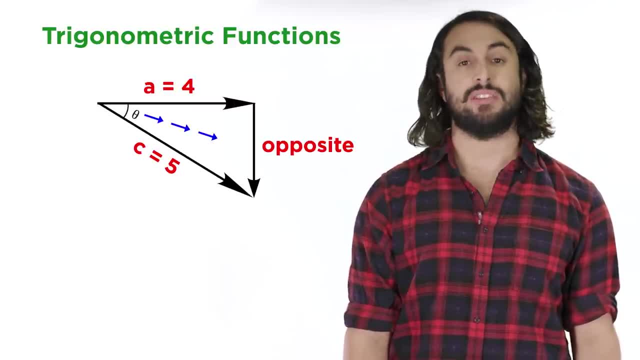 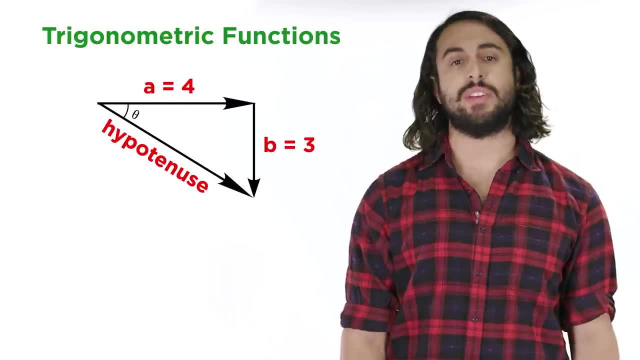 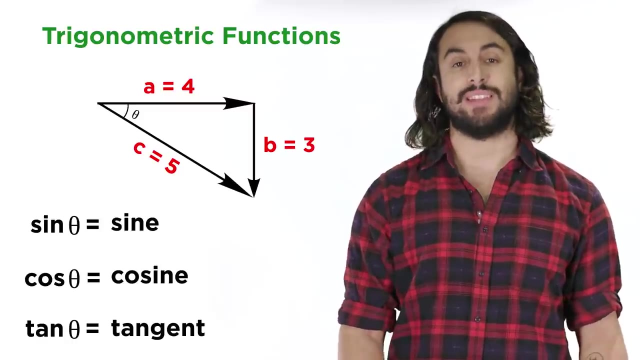 and label the sides of the triangle as opposite: the leg directly opposite the angle adjacent the leg right next to the angle and the hypotenuse, which is always the longest side. We can use the lengths of these sides to find the sine cosine and tangent of this angle. 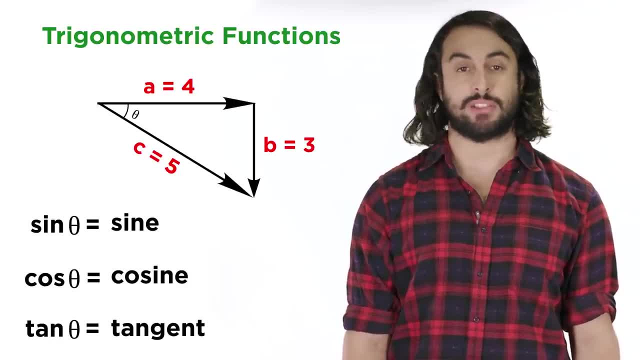 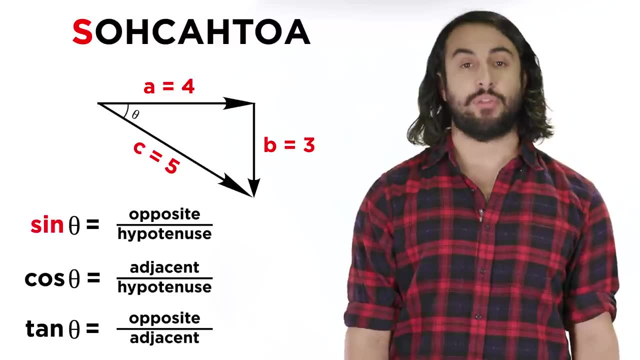 We will cover these functions in more depth in the upcoming mathematics course, But for now all we need to remember is the mnemonic device SOHCAHTOA. Sine theta is equal to opposite over hypotenuse. In this case, that would be three fifths. 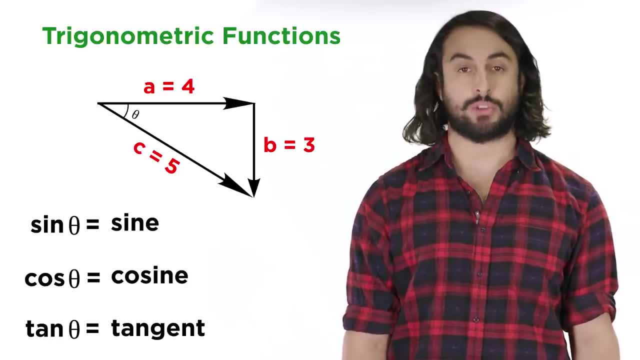 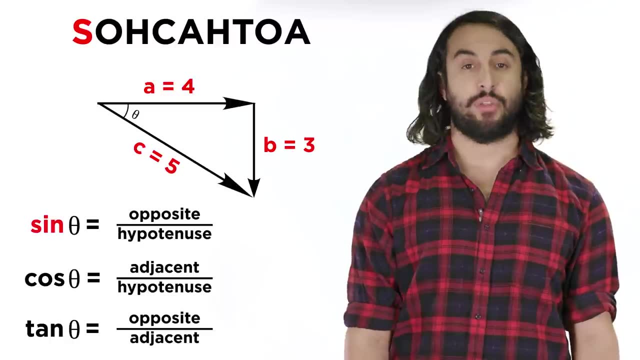 We will cover these functions in more depth in the upcoming mathematics course, But for now all we need to remember is the mnemonic device SOHCAHTOA. Sine theta is equal to opposite over hypotenuse. In this case, that would be three fifths. 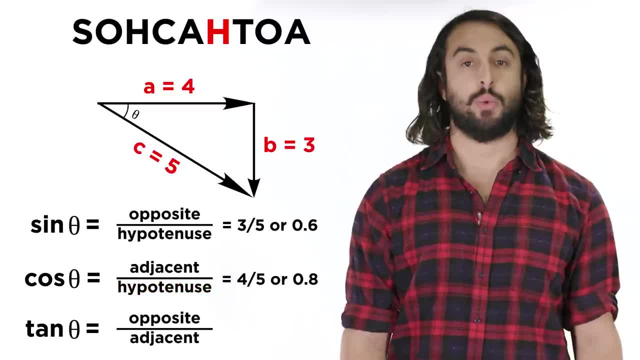 Cosine theta is equal to adjacent over hypotenuse, which here will be four fifths, And tangent theta is opposite over adjacent or three fourths. To solve for theta, we can use any of these equations. Using this one, we can take the inverse. 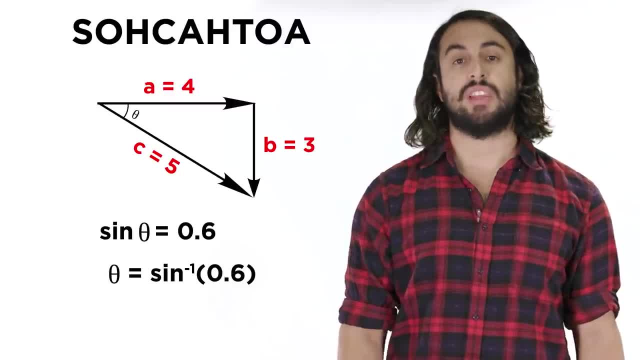 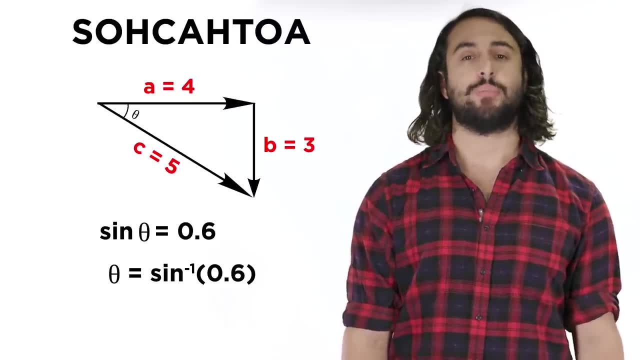 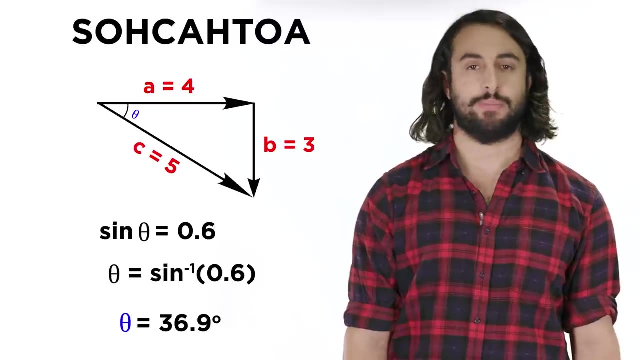 The inverse sine of both sides. That makes theta equal to the inverse sine of three fifths. Just put three over five- or 0.6, into your calculator and press the inverse sine button, which may look like any of these expressions, and we get about 36.9 degrees. 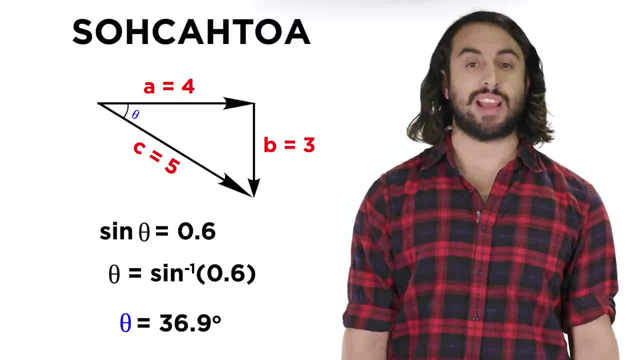 Trigonometric functions like these relate the angles of a right triangle to the lengths of the sides, and we will use them a lot in physics, but it usually won't be more complicated than this, so don't worry too much about it. Also, if you are using a graphing calculator, take a moment to familiarize yourself with 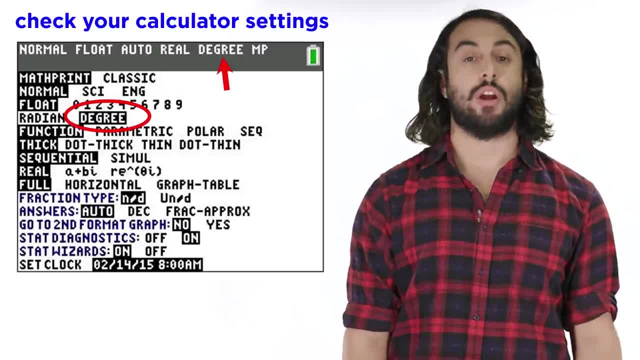 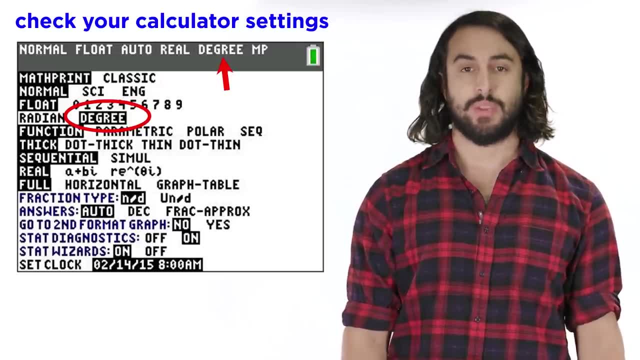 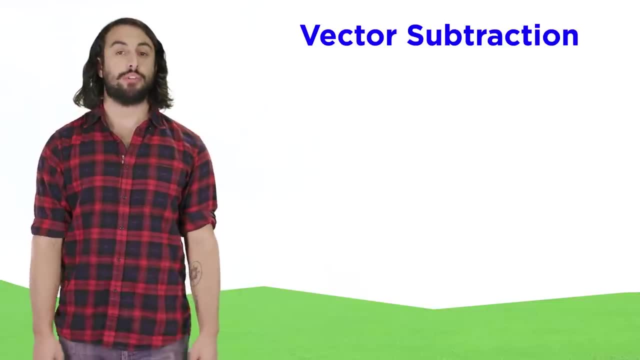 the different settings it uses to report angles, which are degrees and radians. If you are more familiar with degrees, make sure that setting is selected, and we will learn about radians another day. Now that we understand vector addition, let's quickly go through a few other operations. 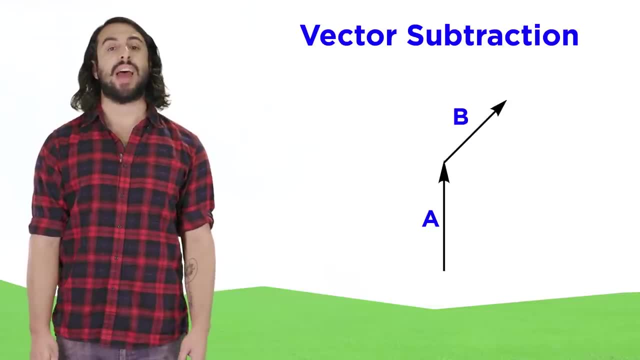 Vector subtraction will be similar to vector addition. Vector subtraction is a function of the vector addition. Vector subtraction is a function of the vector addition. In this case we are subtracting vectors. We will again line them up head to tail, but we will invert the direction of the second. 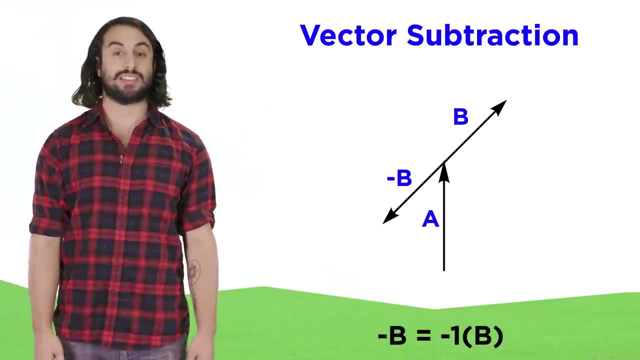 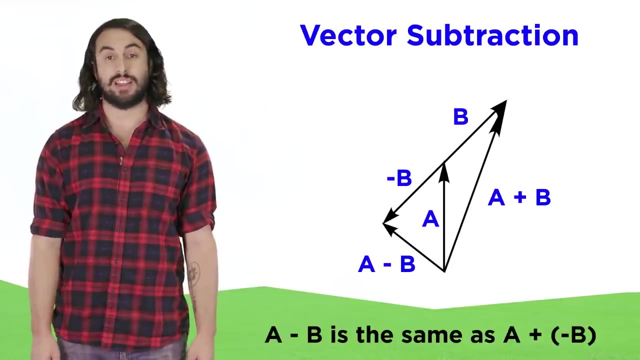 vector. This is the same as multiplying the vector by a scalar of negative one. This way, the magnitude of the vector remains the same, but its direction is reversed. So instead of A plus B, which looks like this, A minus B would look like this, which is essentially: 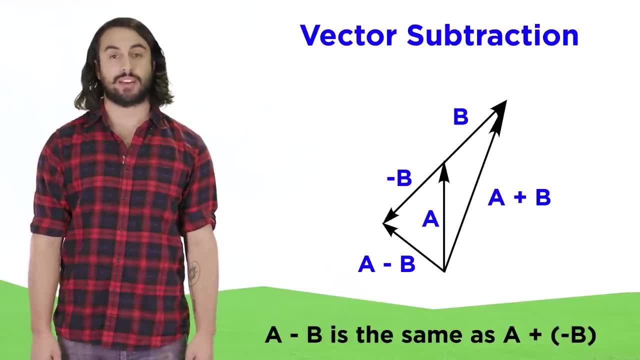 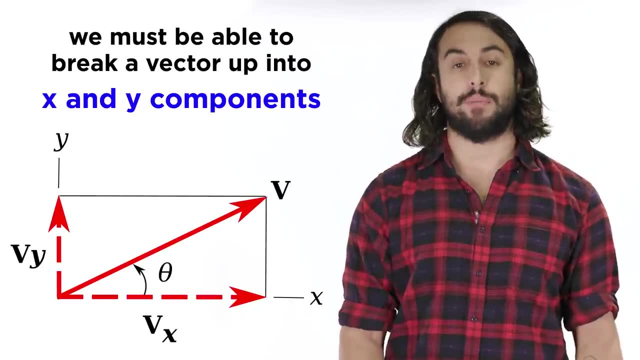 A plus negative B, We find the resultant vector is a constant. that's all there is to it. Another thing we might want to do is break up a vector into X and Y components. This is useful when looking at projectile motion. If a 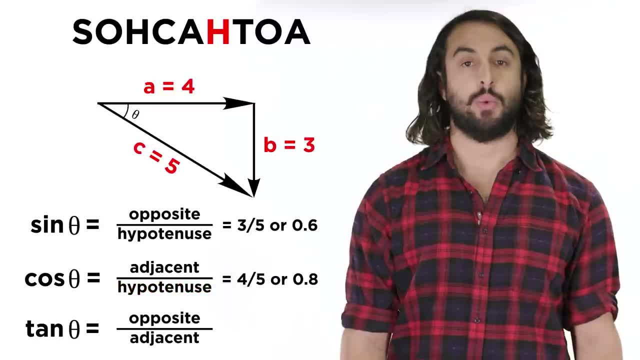 Cosine theta is equal to adjacent over hypotenuse, which here will be four fifths, And tangent theta is opposite over adjacent or three fourths. To solve for theta, we can use any of these equations. Using this one, we can take the inverse of theta. 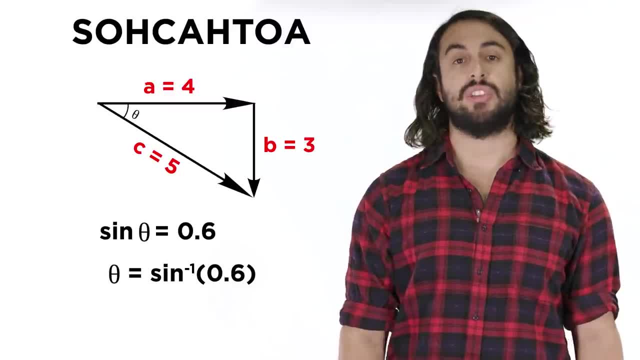 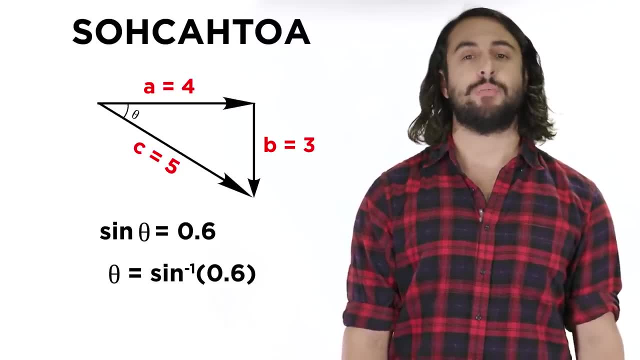 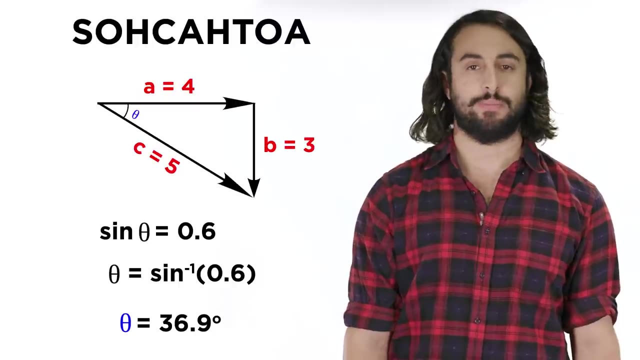 This is the inverse sine of both sides. That makes theta equal to the inverse sine of three fifths. Just put three over five- or 0.6, into your calculator and press the inverse sine button, which may look like any of these expressions, and we get about 36.9 degrees. 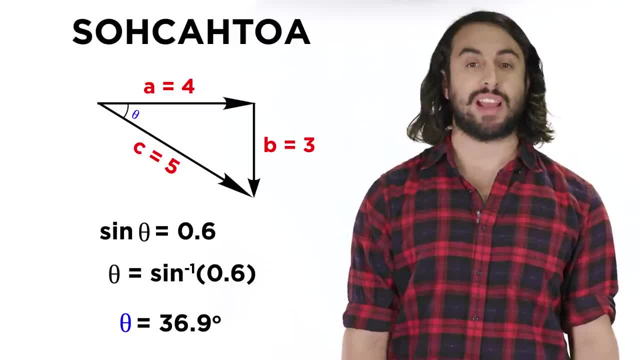 Trigonometric functions like these relate the angles of a right triangle to the lengths of the sides, and we will use them a lot in physics, but it usually won't be more complicated than this, so don't worry too much about it. Also, if you are using a graphing calculator, take a moment to familiarize yourself with 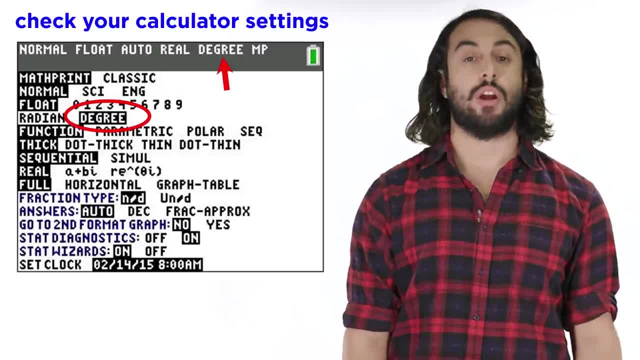 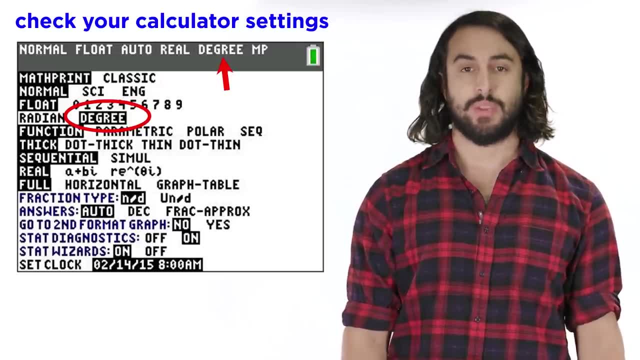 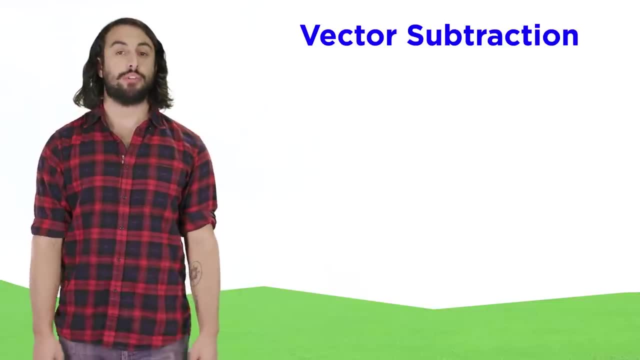 the different settings it uses to report angles, which are degrees and radians. If you are more familiar with degrees, make sure that setting is selected, and we will learn about radians another day. Now that we understand vector addition, let's quickly go through a few other operations. 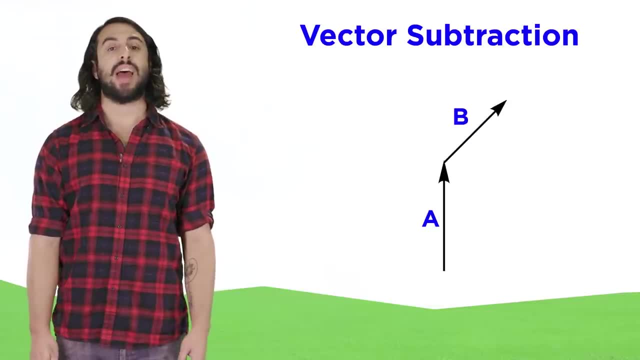 Vector subtraction will be similar to vector addition. Vector subtraction is a function of vector addition. Vector subtraction is a function of vector addition. When we are subtracting vectors, we will again line them up head to tail, but we will invert the direction of the second vector. 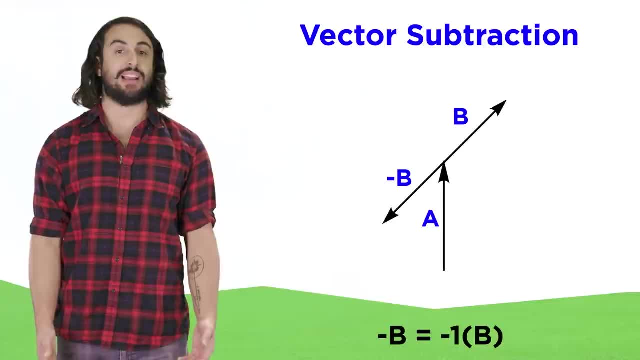 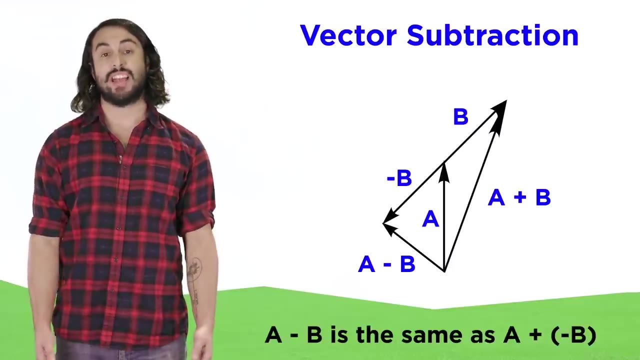 This is the same as multiplying the vector by a scalar of negative one. This way, the magnitude of the vector remains the same, but its direction is reversed. So instead of A plus B, which looks like this, A minus B would look like this, which is essentially: 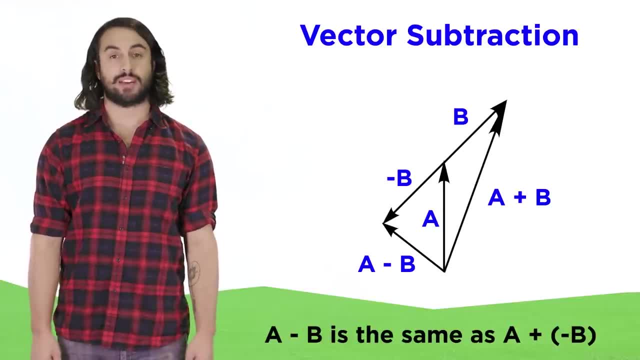 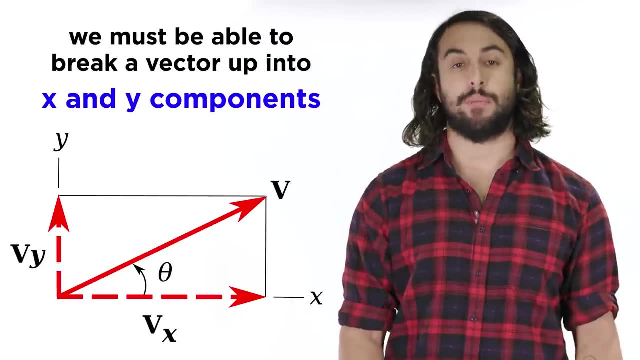 A plus negative B, We find the resultant vector B is the same A plus B resultant vector, and that's all there is to it. Another thing we might want to do is break up a vector into X and Y components. This is useful when looking at projectile motion. 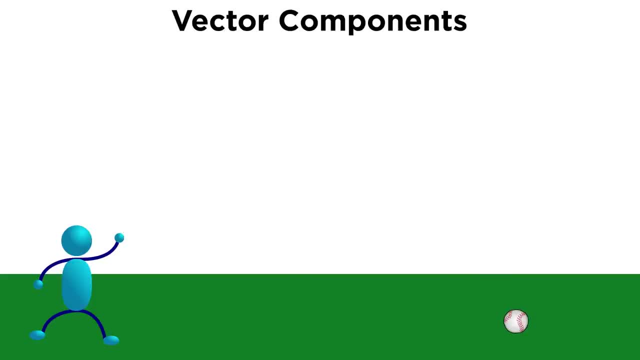 If a ball is thrown at an angle, its velocity can be represented with a vector, But because gravity is operating on the ball in the Y direction, pulling it down to the earth, we will want to be able to separate its vertical motion from its horizontal motion. 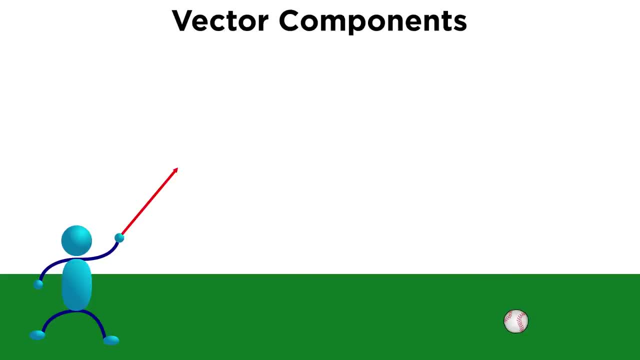 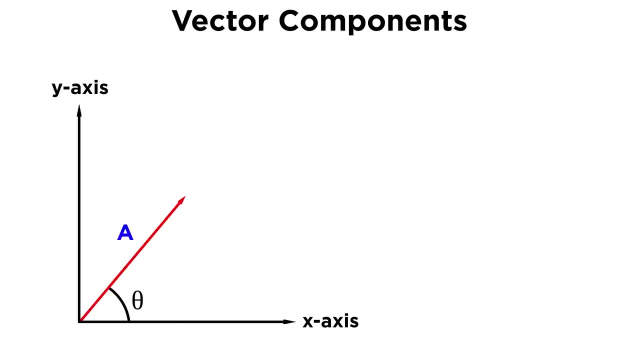 ball is thrown at an angle, its velocity can be represented with a vector. but because gravity is operating on the ball in the Y direction, pulling it down to the earth, we will want to be able to separate its vertical motion from its horizontal motion, so we can take this vector and split it up into components. 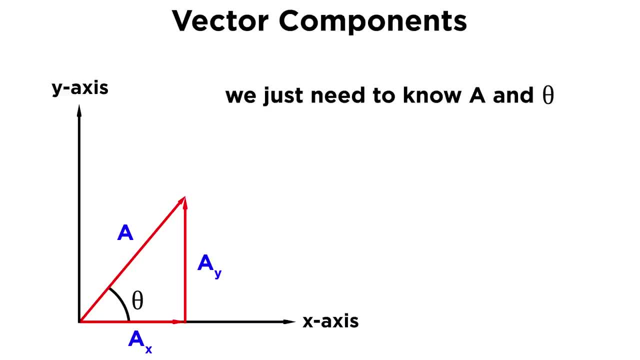 All we need to know is the magnitude of the vector and its angle from the horizontal. Then we can use trigonometry to find the lengths of the legs of a hypothetical right triangle. Sine of theta gives us opposite over hypotenuse, and cosine theta gives us adjacent over hypotenuse. On both of these we can. 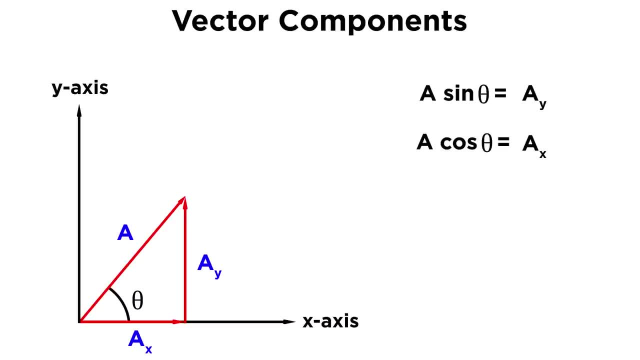 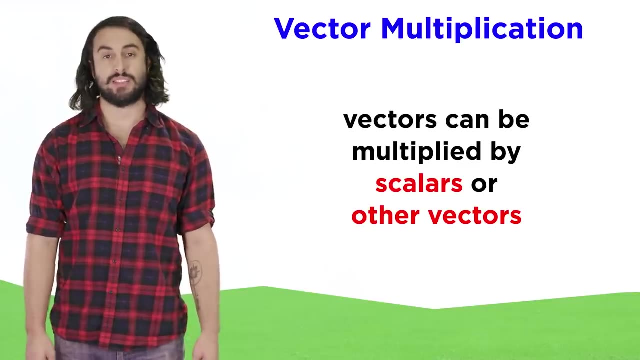 evaluate the trig function and multiply both sides by the hypotenuse, which is the value we know, to get the legs of the triangle, Which will be the X and Y components of the vector. We will see this in more detail later. Vectors can also be multiplied by scalars or other vectors. 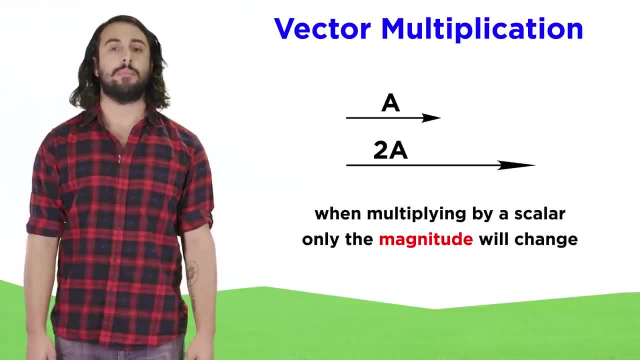 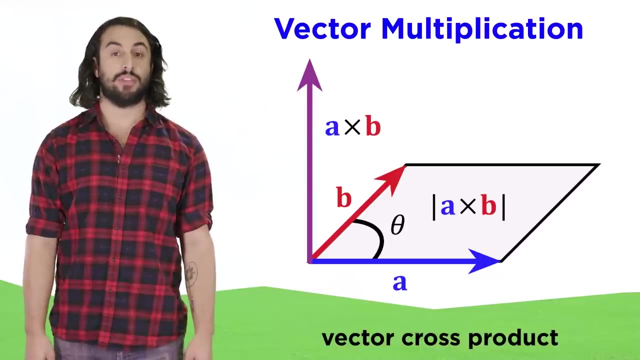 When multiplying a vector by a scalar, we will simply multiply the magnitude of that vector by the scalar, while keeping the direction the same. So if multiplying this vector by two, its length will double. Two vectors can also be multiplied, but that will be more complicated, so we will go over that. 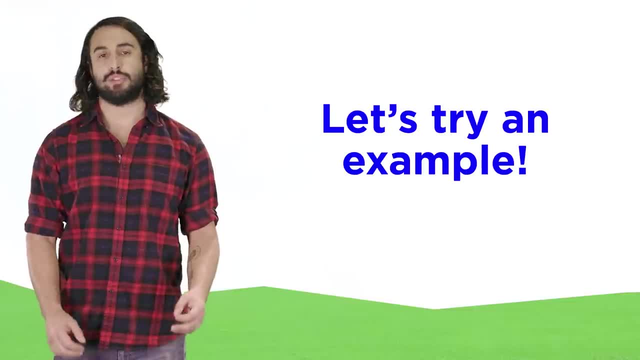 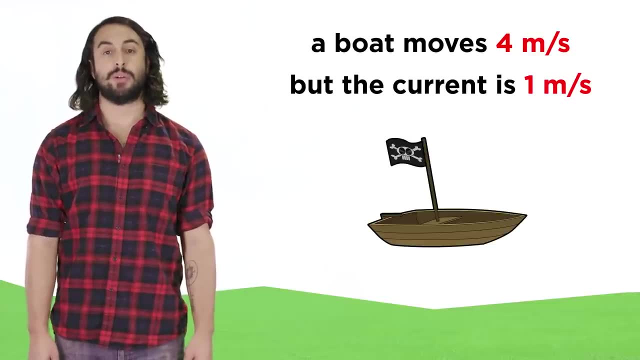 another time. Let's try one example to make sure we can do these kinds of calculations. Say you are in a boat traveling across a river and the boat typically moves at four meters per second in still water, but the current is pushing you downstream at a rate of one meter per second. 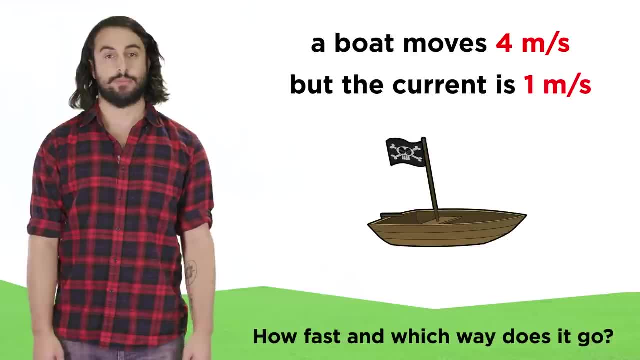 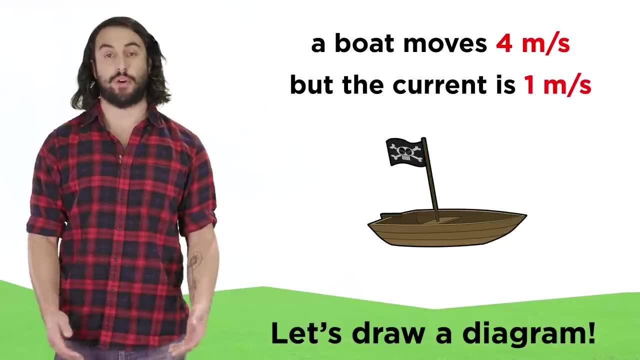 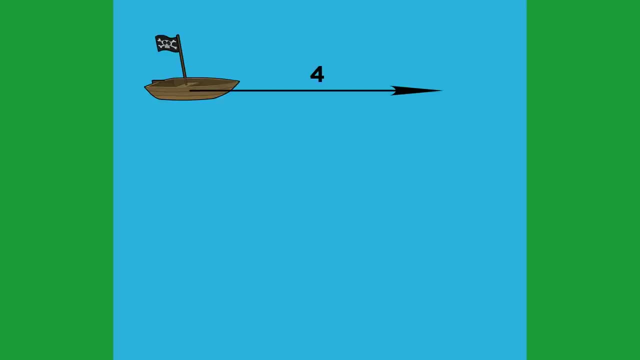 What is the speed and direction of the boat? To answer this and almost any other problem we study in physics, it is best to draw a diagram first. Here's a top-down view of the river and the boat. Let's draw a vector that is horizontal with a magnitude of four. We then need 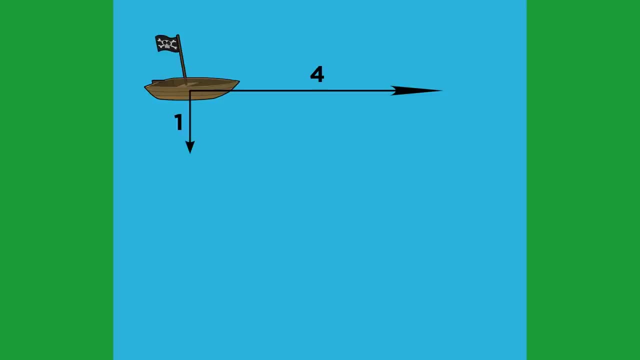 another vector to represent the current. that will point straight down and have a magnitude of 1.. To find out the speed and direction of the boat, we have to add these vectors together. In order to do this, we can move the vector that. 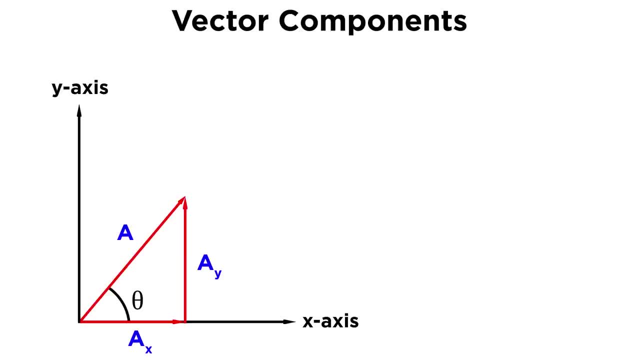 so we can take this vector and split it up into components. All we need to know is the magnitude of the vector and its angle from the horizontal. Then we can use trigonometry to find the lengths of the legs of a hypothetical right triangle. 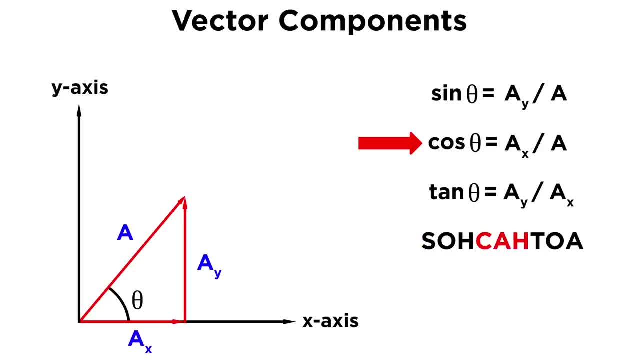 Sine of theta gives us opposite over hypotenuse and cosine theta gives us adjacent over hypotenuse. On both of these we can evaluate the trig function and multiply both sides by the hypotenuse, which is the value we know to get the legs of the triangle, which will be the X and Y. 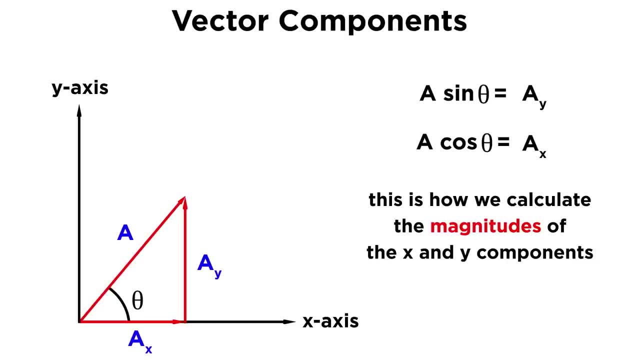 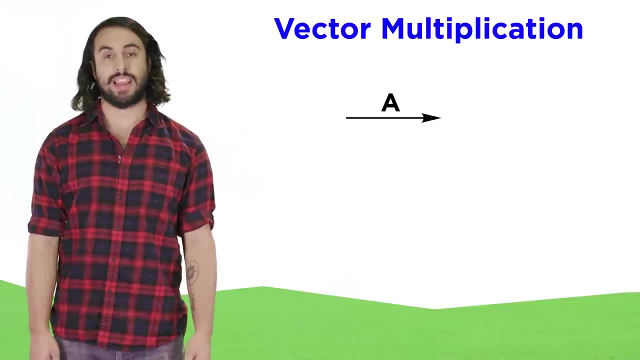 components of the vector. We will see this in more detail later. Vectors can also be multiplied by scalars or other vectors. When multiplying a vector by a scalar, we will simply multiply the magnitude of that vector by the scalar, while keeping the direction the same. 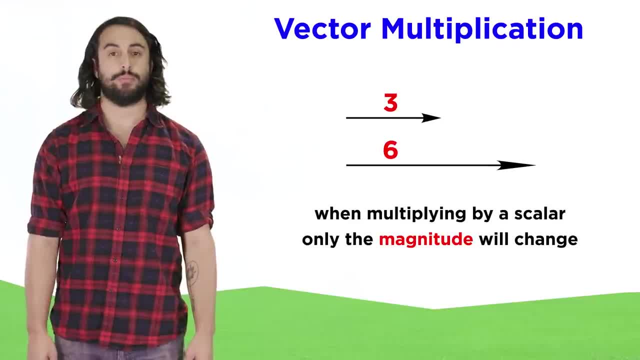 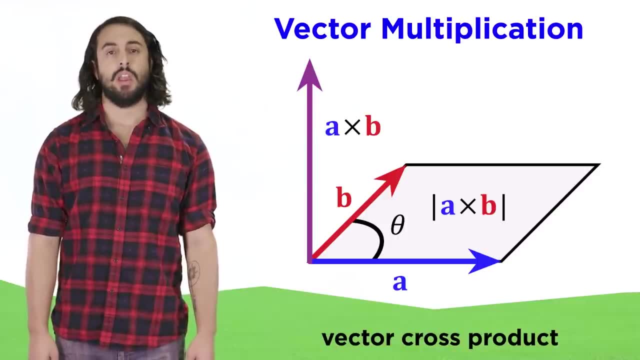 So if, multiplying this vector by two, its length will double. Two vectors can also be multiplied, but that will be more of a problem. We will see this in more detail later. Let's try one example to make sure we can do these kinds of calculations. 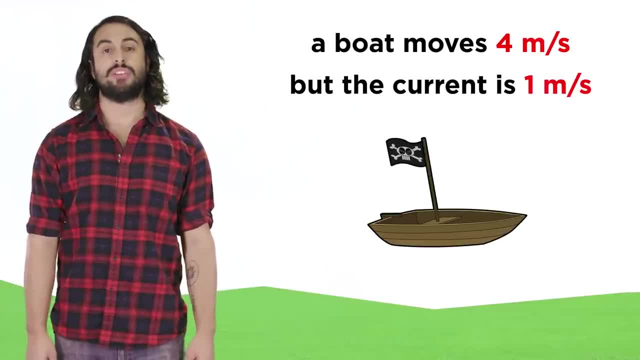 Say you are in a boat traveling across a river and the boat typically moves at four meters per second in still water, But the current is pushing you downstream at a rate of one meter per second. What is the speed and direction of the boat? 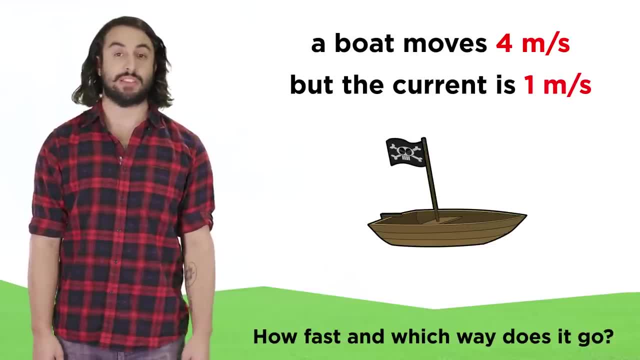 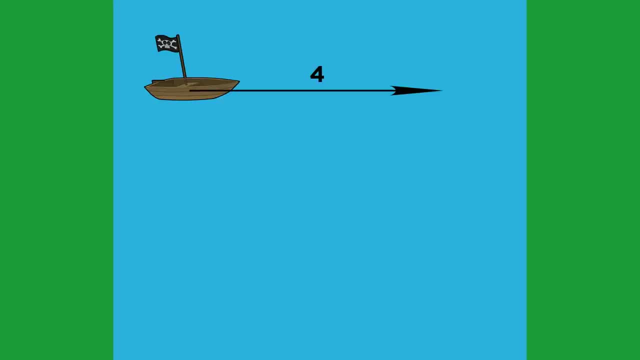 To answer this and almost any other problem we study in physics, it is best to do the diagram first. Here is a top-down view of the river and the boat. Let's draw a vector that is horizontal with a magnitude of four. We then need another vector to represent the current. 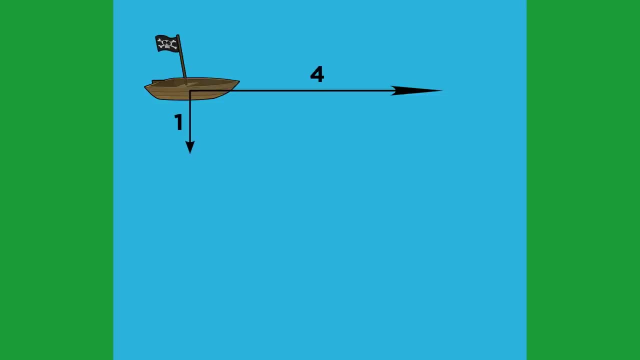 That will point straight down and have a magnitude of one. To find out the speed and direction of the boat. we have to add these vectors together. In order to do this, we can move the vector that represents the current over here, so that we are adding head to tail. 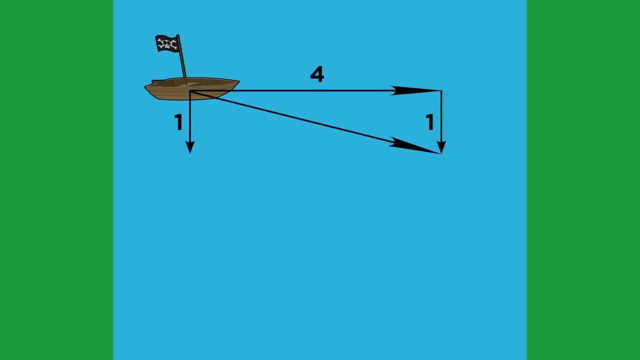 And then find the resultant vector. Or we could have left it where it was, made a rectangle using the two vectors and then just drawn the diagonal. Either way, this vector sum will have a magnitude of root seventeen. To find the angle from the horizontal we can use any trig function we like.